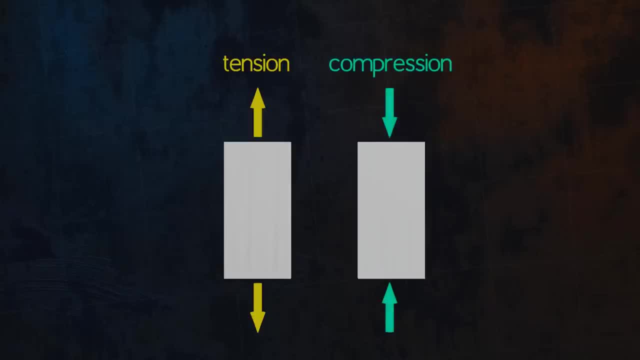 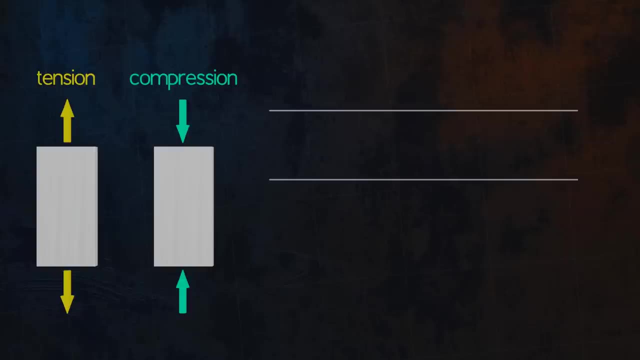 But what about the compressive direction? For ductile materials like mild steel, the yield and ultimate strengths are very similar in the tensile and the compressive directions. Tensile tests are usually easier to carry out than compression tests, and so compression tests aren't often performed for these materials. 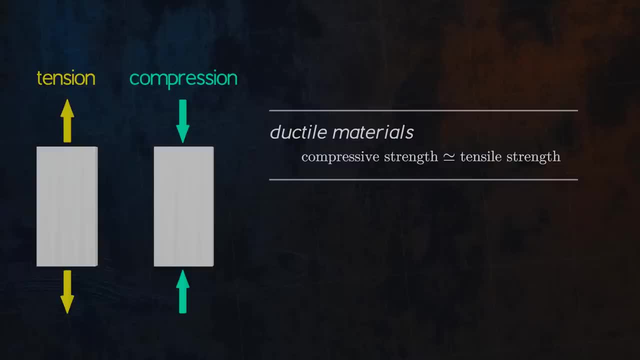 For brittle materials like concrete and ceramics, however, the material strength is much larger in compression than in tension. I will talk about why this is the case later on in the video. First, let's look at some examples of strength values for a few different materials. 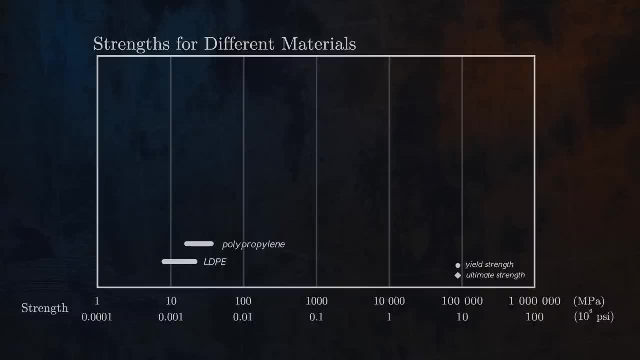 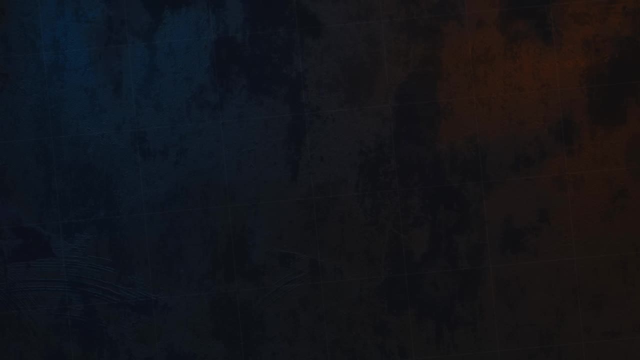 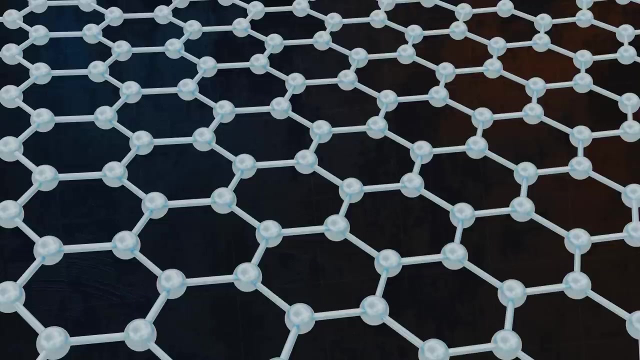 Tensile yield strengths are shown for ductile materials and ultimate compressive strengths are shown for brittle materials. Graphene is the strongest material to have ever been tested. It is a two-dimensional material made up of a single layer of carbon atoms arranged in a hexagonal lattice and linked by strong covalent bonds. 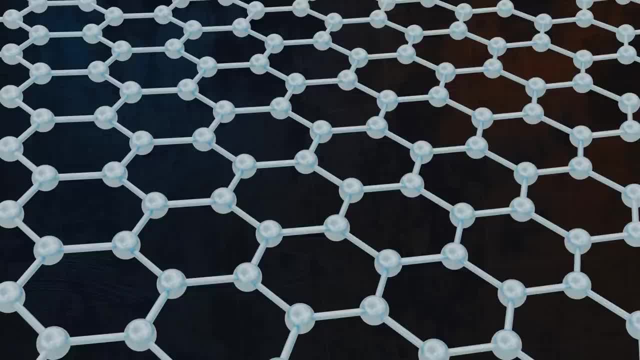 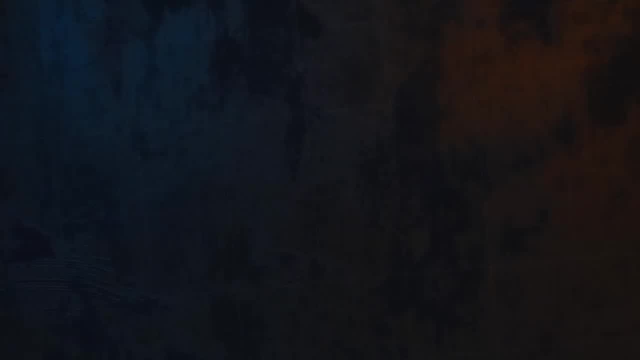 Defect-free graphene has an ultimate tensile strength of up to 130 gigapascals or 19,000 kA. I've mentioned material ductility a few times in this video, so now is probably a good time to define it properly. 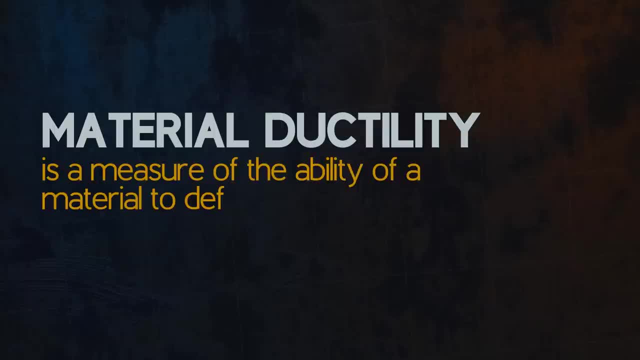 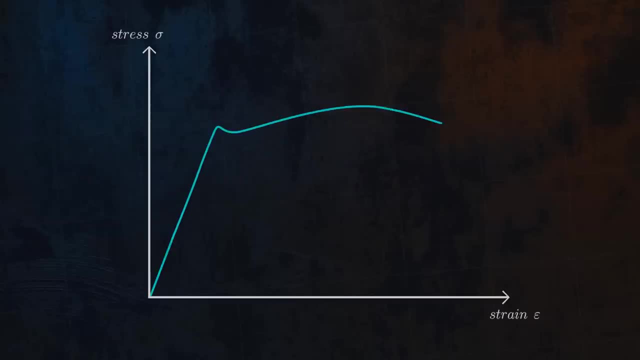 Ductility is a measure of the ability of a material to deform plastically before fracture. Let's return to our stress-strain curve. Materials which undergo large amounts of plastic deformation before they break are called ductile materials. These materials fracture at very large strains. 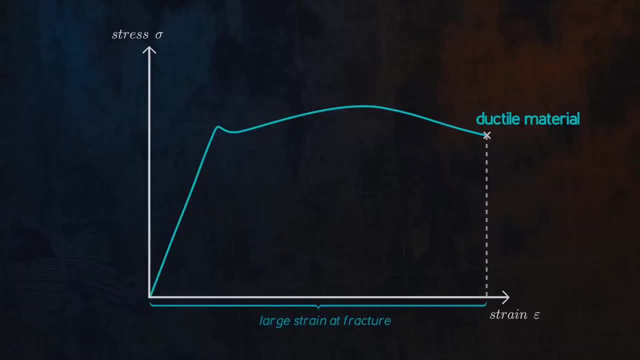 Mild steel and gold are examples of very ductile materials. Materials which fracture at very low strains with little to no plastic deformation are said to be brittle. Glass and ceramics like porcelain are examples of brittle materials Because they don't deform plastically. the concept of yield strength is irrelevant for brittle materials. 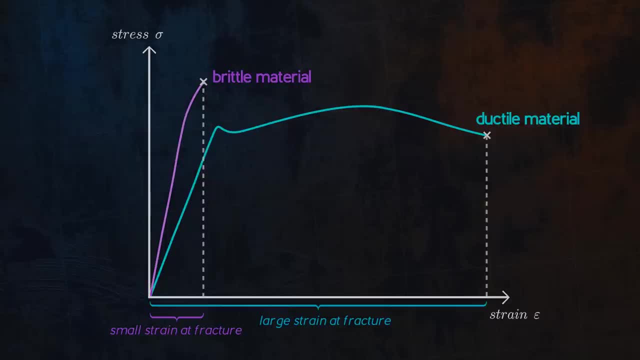 There is no defined transition point between ductile and brittle behavior. Typically, a material which has a strain at fracture of less than 5% is considered to be brittle. Now that we have covered what ductile and brittle materials are, let's return to the question of why brittle materials are much stronger in compression than in tension. 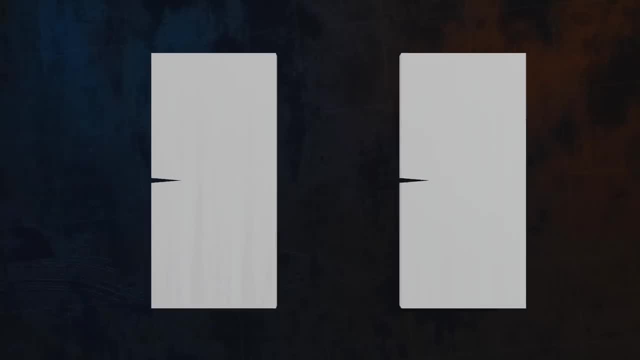 There are two factors at play. The first factor is that tensile loads tend to encourage the formation and propagation of cracks, whereas compressive loads do not, as illustrated here. The second factor is that in brittle materials, very little or no plastic deformation occurs. 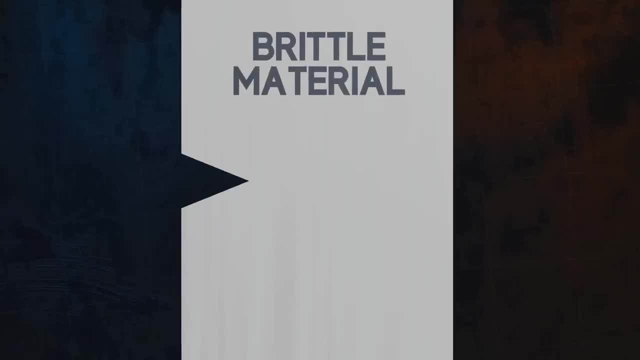 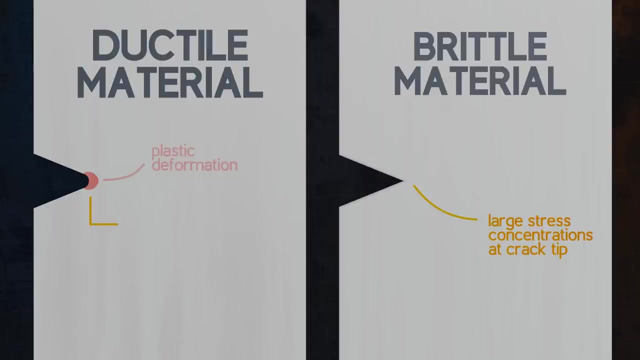 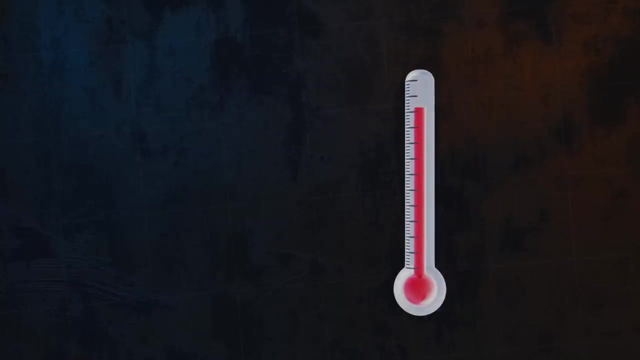 to redistribute stresses at existing flaws. This means that large stress concentrations build up at the cracked tip, resulting in fracture In ductile materials, plastic deformation occurs, which relieves these localized stresses. In the case of metal, ductility can be dependent on temperature. 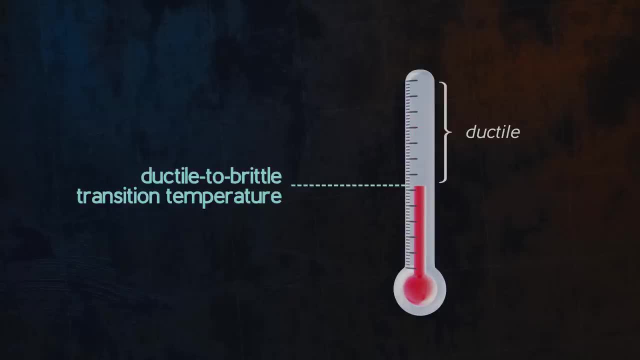 A lot of different types of steel, for example, are ductile at room temperature but become brittle when the temperature drops to below the ductile to brittle transition temperature. This transition temperature is an important design consideration because ductile failure is normally preferred to brittle failure. 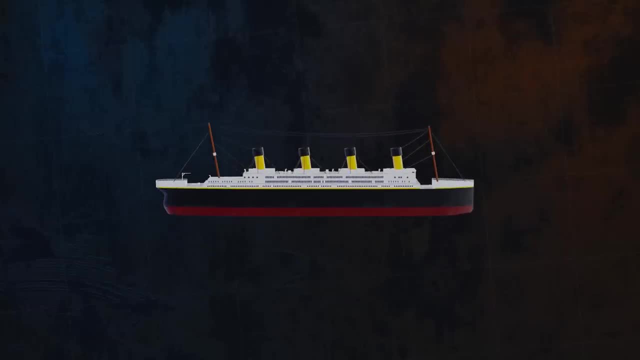 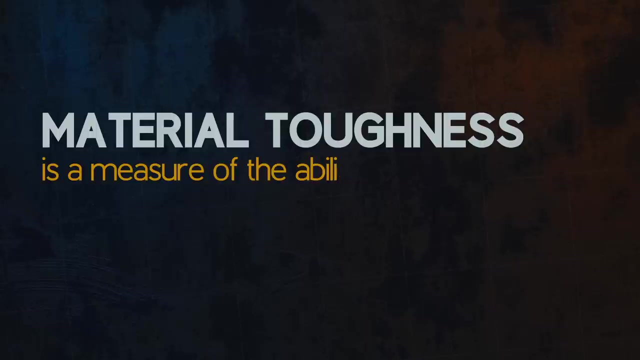 One very famous example of brittle failure is the Titanic. The icy waters of the North Atlantic are thought to have caused the steel of the ship's hull to drop below its ductile-to-brittle transition temperature, resulting in catastrophic brittle fracture. Toughness is the ability of a material to absorb energy up the fracture. 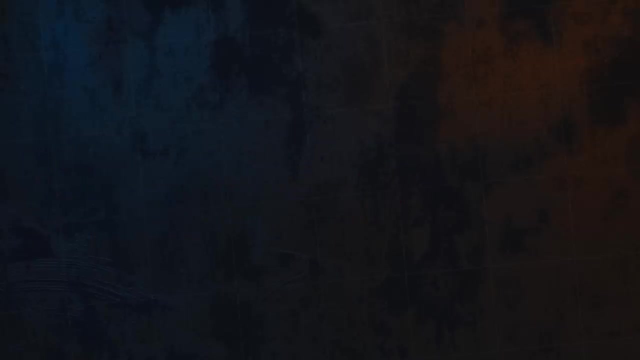 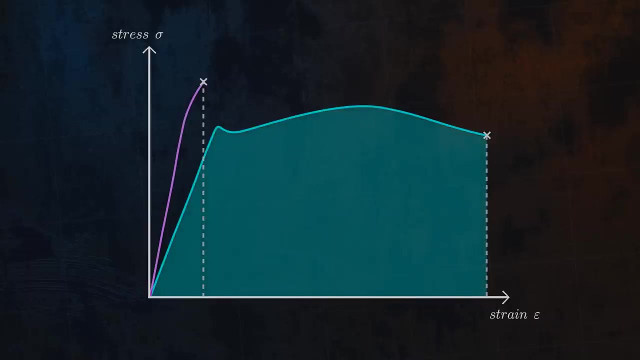 It can be calculated as the area under the stress-strain curve. If the area under the stress-strain curve is large, the material will have high toughness and so will be able to absorb a large amount of energy before fracturing. For a material to have high toughness, it should have a good balance of both ductility and strength. 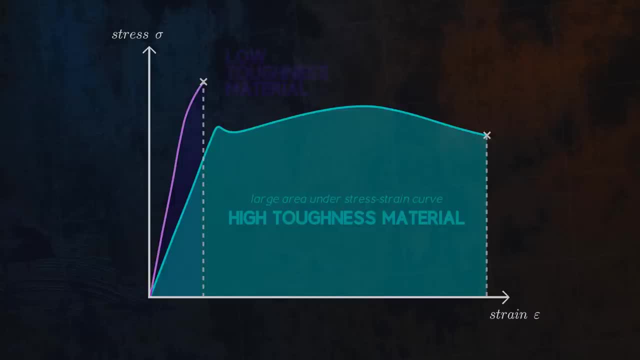 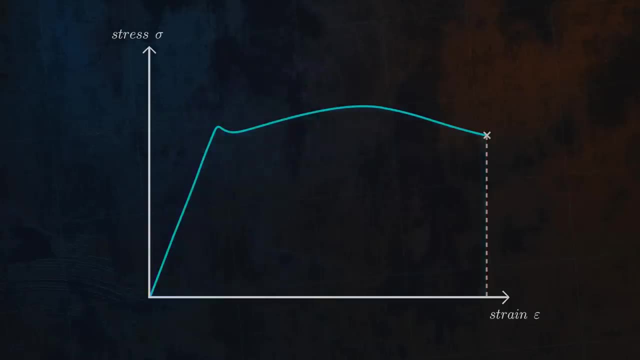 Low-strength materials and brittle materials tend to have low toughness. a A related property is resilience, which is the ability of a material to absorb energy when deforming. elastically, It corresponds to the area under the stress-strain curve, but only within the elastic region. 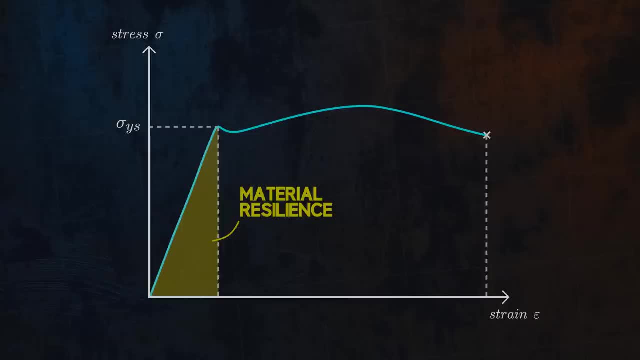 Materials with high resilience are well suited for applications where plastic deformation is to be avoided. To summarize, the yield strength of a material defines the stress at which it begins to deform plastically. The ultimate tensile strength defines the maximum stress which is reached during the